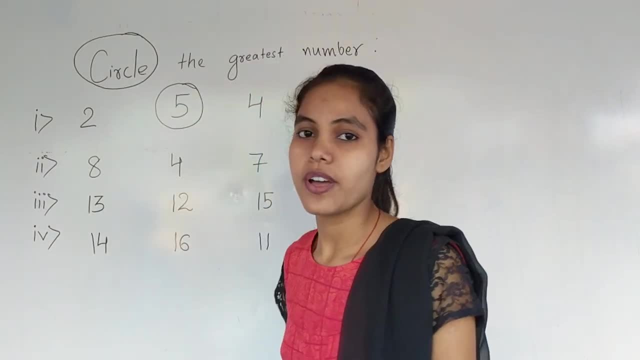 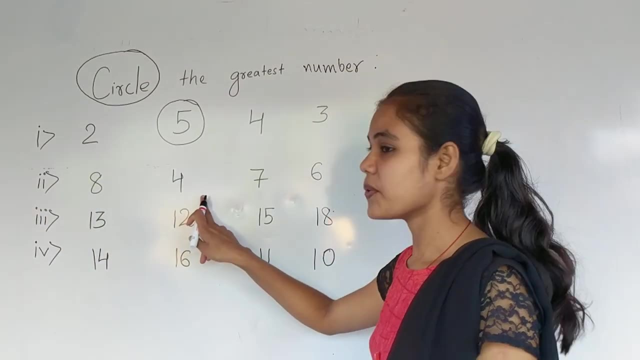 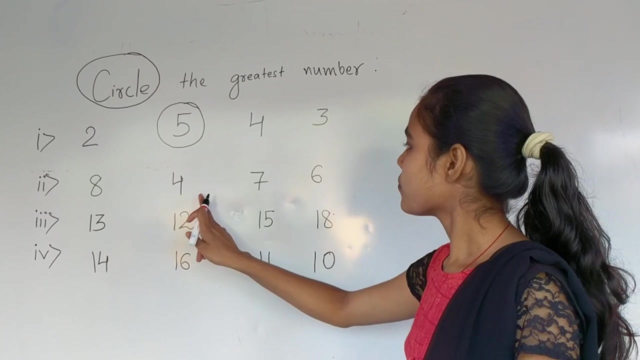 5 is Circle, We will circle 5.. Next number: 2.. 8,, 4,, 7 and 6.. Here the smallest number is 4.. Bigger than 4 is 6.. Bigger than 6 is 7.. 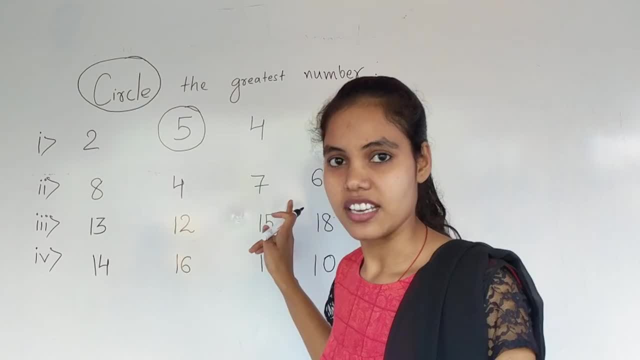 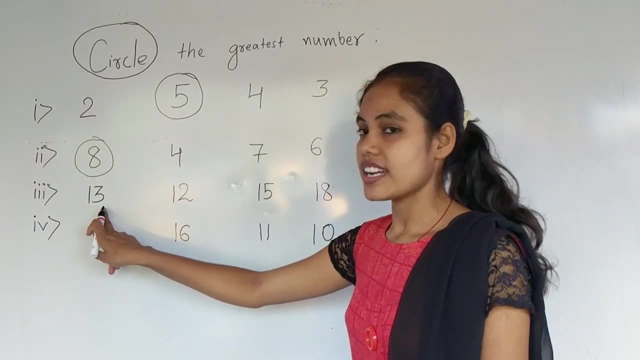 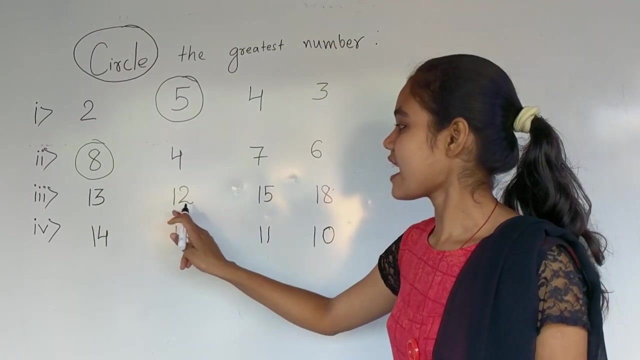 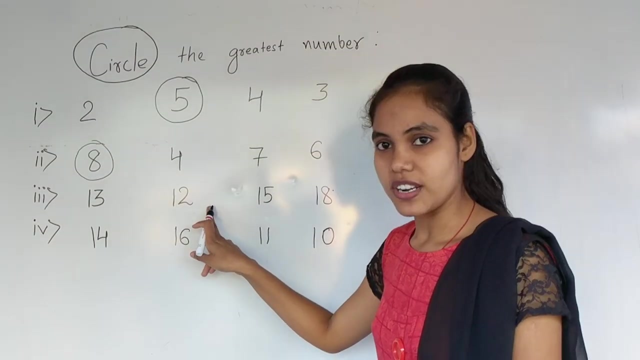 And 8 is the biggest number in this line. So 8 is Circle Number 3.. 13,, 12,, 15 and 18.. In this line, 12 is a small number, Smallest number, 13 is bigger than 15.. 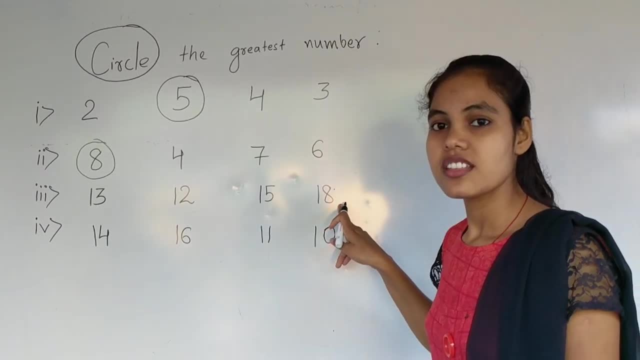 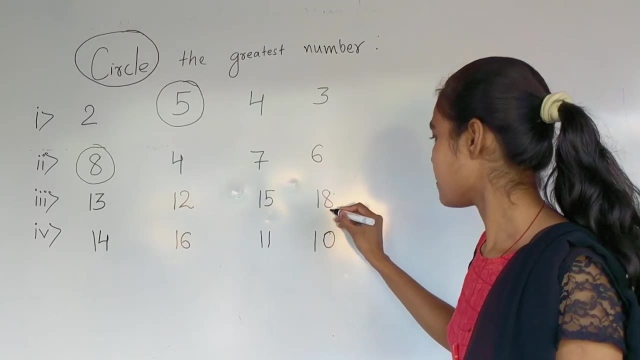 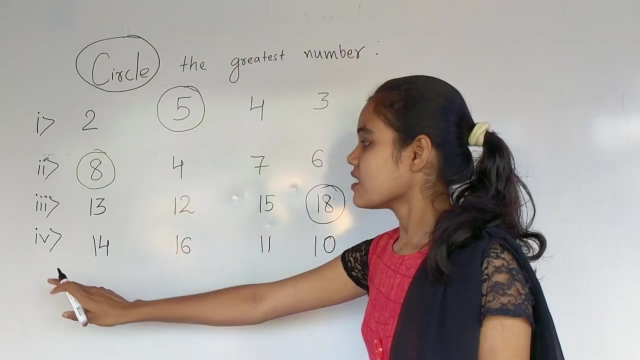 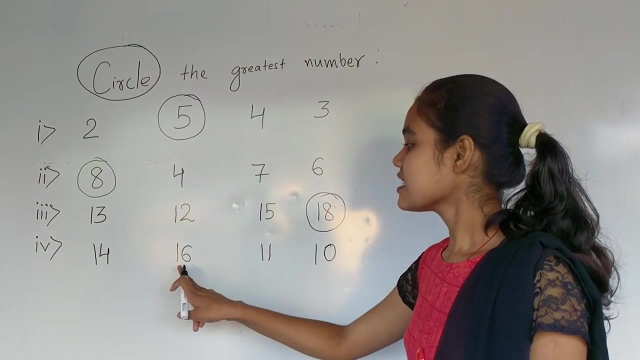 15 is bigger than that And 18? Bigger than that, Bigger than that. So 18 is Biggest, Biggest number Circle, the 18. Number 4.. It is my last number: 14,, 16,, 11 and 10.. 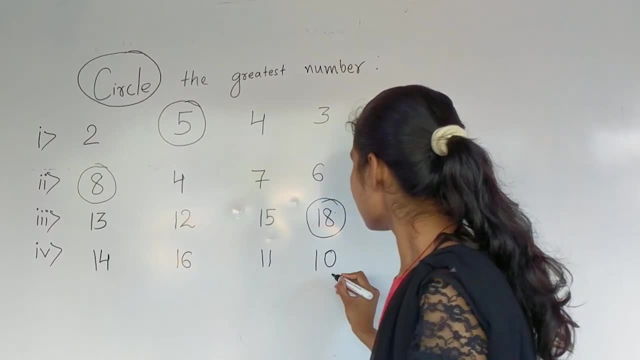 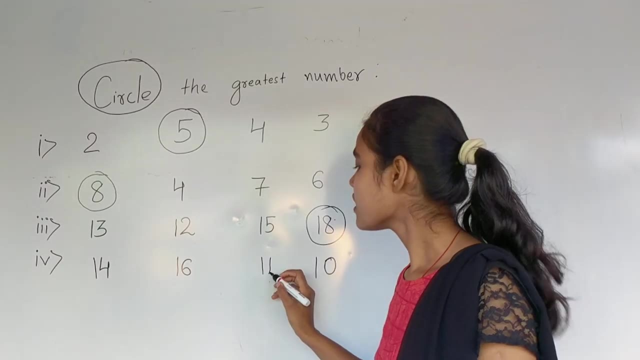 10 is smaller, 10 is the biggest, 11 is bigger, 14 is bigger than that And 16 is biggest, So 16. Circle the number 16.. Here we have said bigger. to explain: Bigger means greatest. 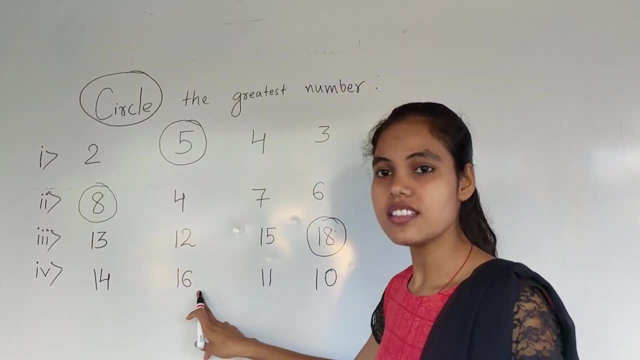 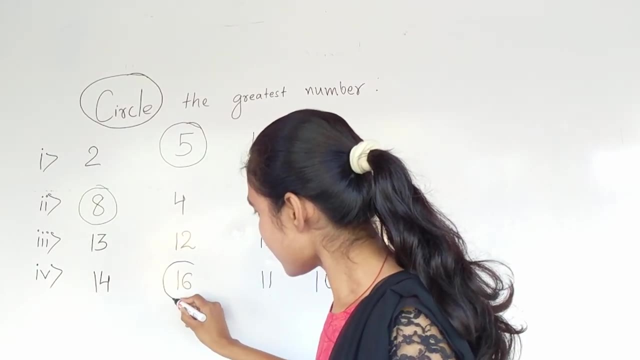 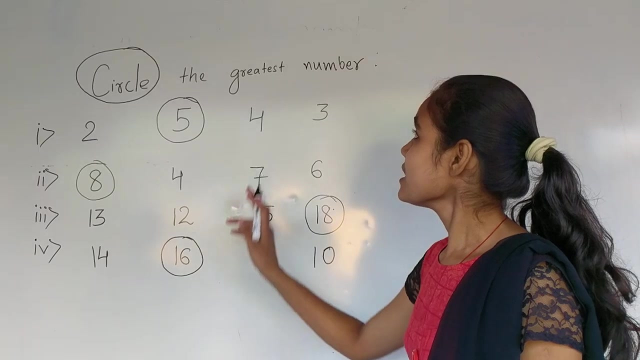 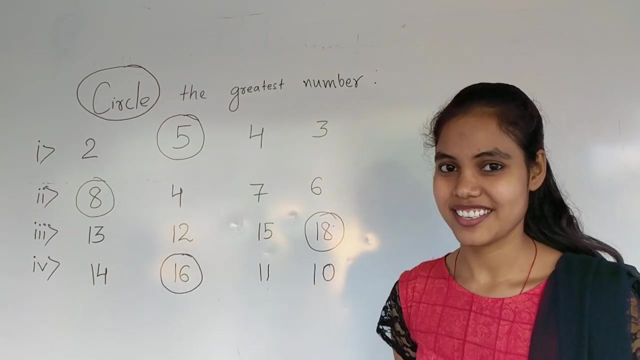 Okay, thank you, Goodbye, See you in the next video, Bye, Bye, Bye, Bye.